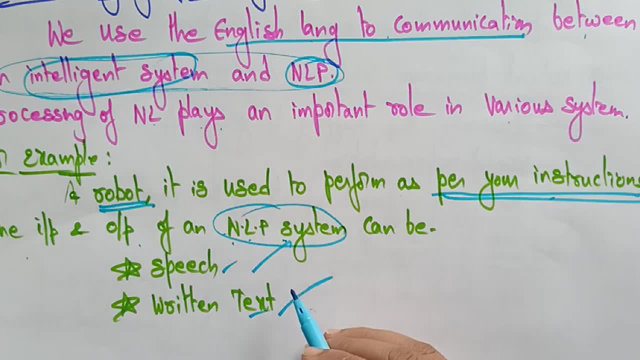 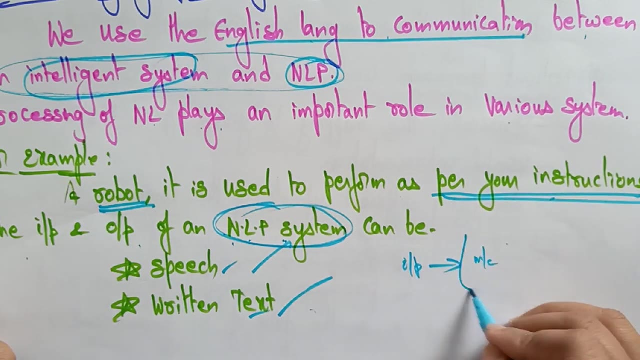 has to become how the input is. Everything will be given to the machine in the way of natural language process. okay, That is a natural language processing. How it is going to, it is giving the input and here in between, it going to be converted into machine language and the system can understand and gives the output, which can be in the form of English language, to communicate. Okay, The user can be. it is, after converting it, just like English language. Giving the input is just like a language. So this is a natural language processing. Okay, This is a natural language processing Cool. 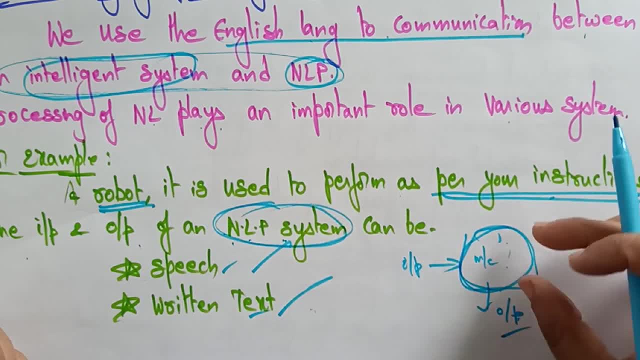 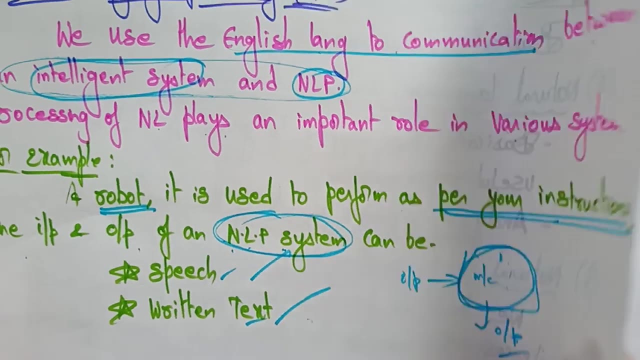 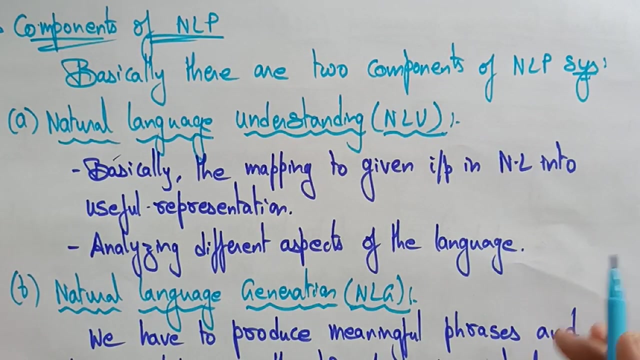 just like english language, but internally it everything will be converted into machine language. so here the natural language processor, uh uh, is going to give the instructions, uh, the input, like speech and written text, everything to the system. what are the components of the natural language processor? basically, there are two components of natural language processor. 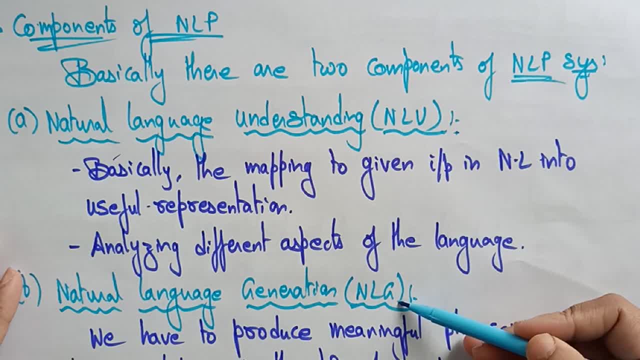 one is the natural language understanding and natural language generation. why i'm calling this two as a components? first thing is you need to understand the concept. okay, the natural language understanding, what is a problem, what are the inputs and what we need to be get. so, after finding, 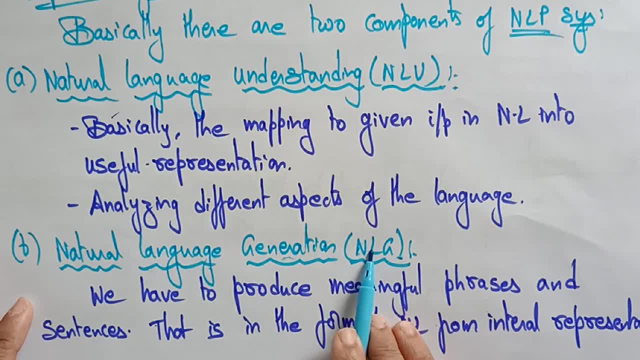 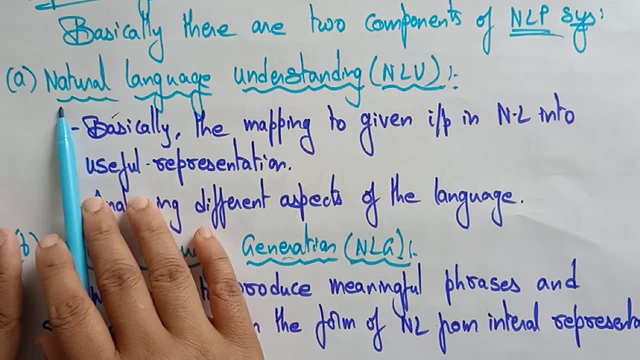 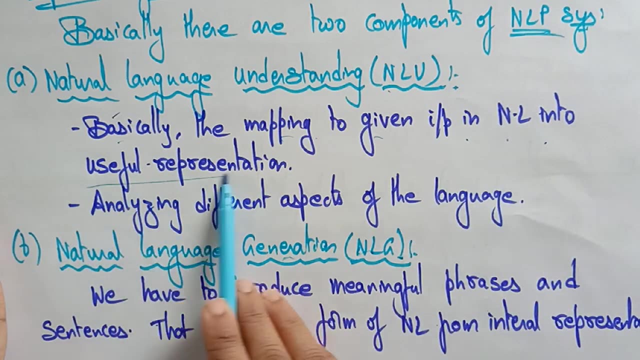 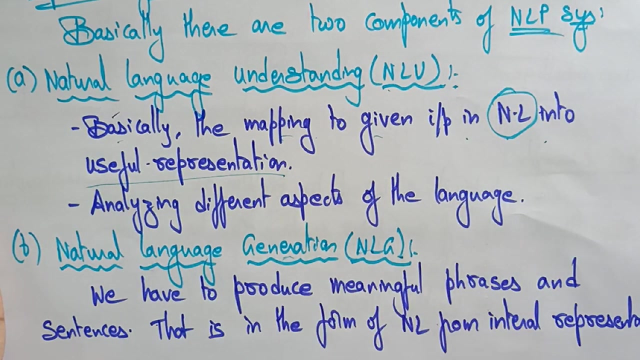 the complete view. the next is natural language generation. then it has to start the work so that the machine can work okay. so now let's see this natural language understanding, basically the mapping to give input in natural language into useful representation, whatever the mapping that you are giving input to the natural language which are represented in a, into some. 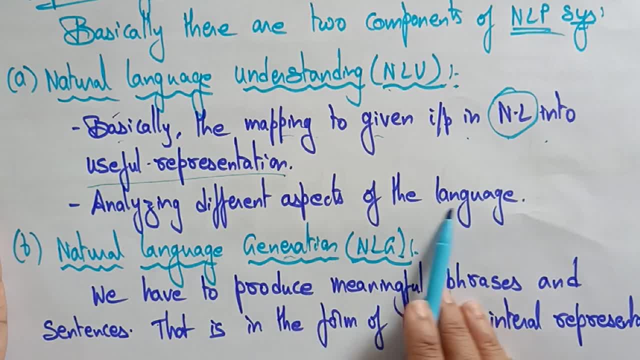 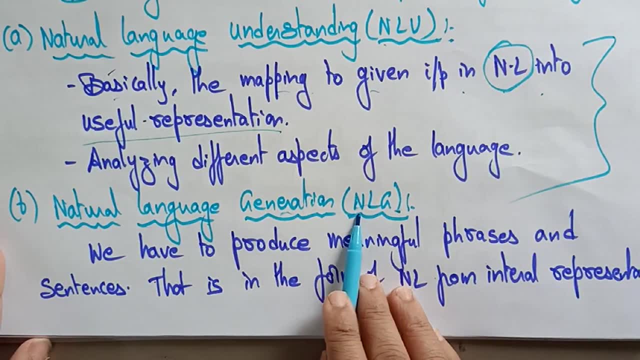 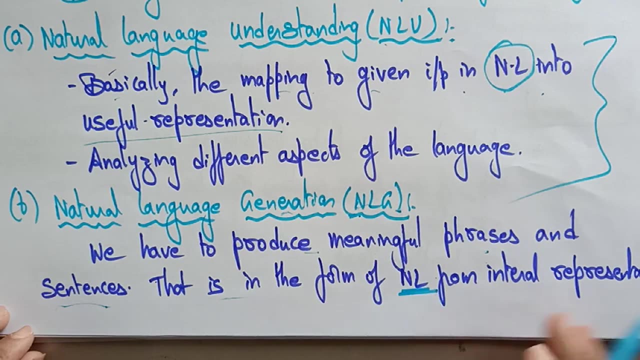 useful representation, like analyzing the different aspects of the language. so it's just the concept of understanding the problem. next, natural language generation. we have to produce the meaningful phrases and sentence that is, in the form of natural language language from internal representation, as this process involves text planning. 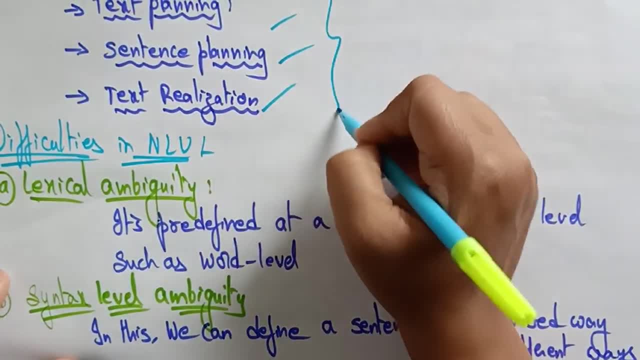 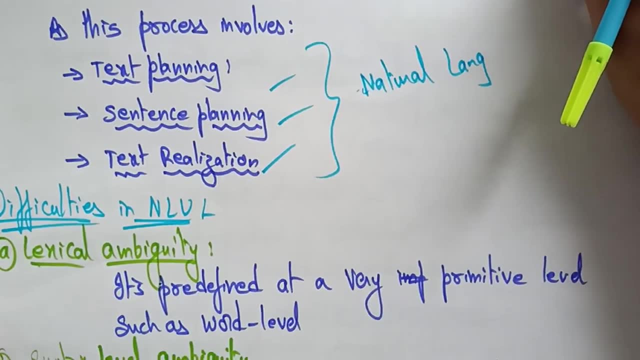 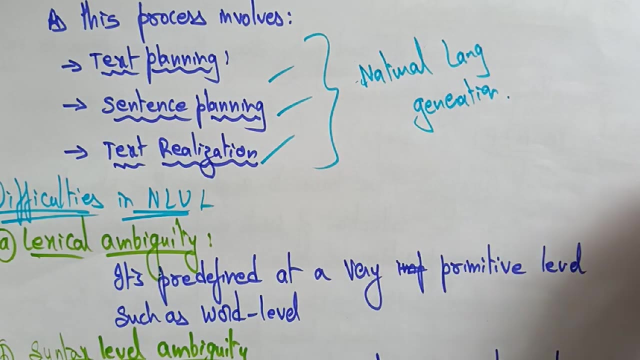 sentence planning: test realization. everything is comes under the natural language generation, natural natural language generation. okay, so it is going to produce a meaningful phrases and the sentence. like text planning, sentence planning, text realization. so in the text planning you are going to plan what are the text that is involved and what are the some words that are present. and next, 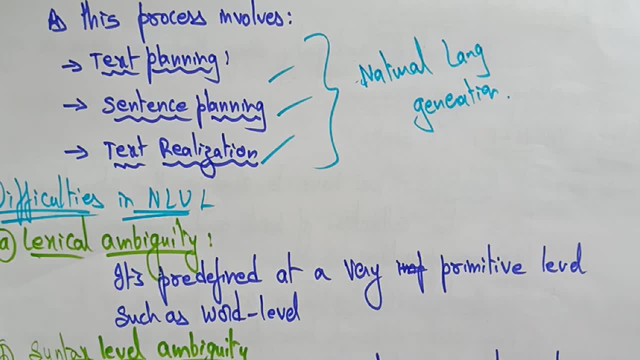 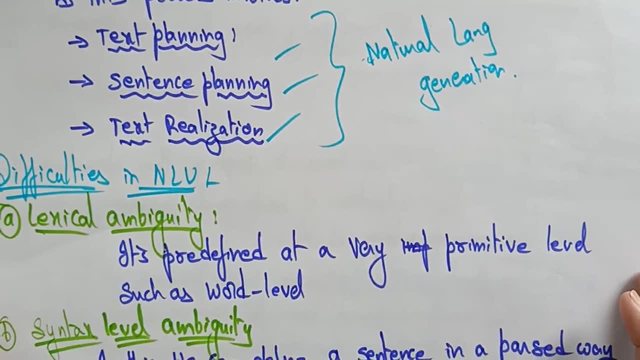 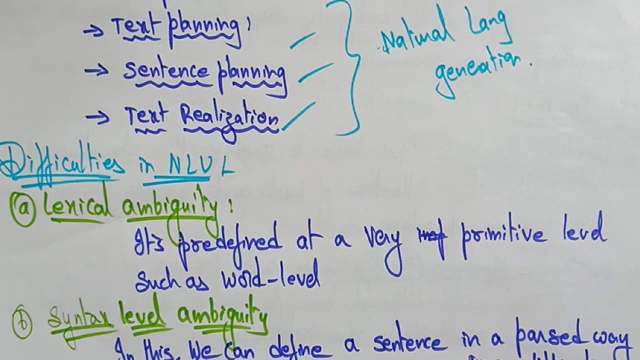 the sentence planning, you have to make it frames and after that the text has to be realized by the machine. this is a way of generating the natural language. now let's see the difficulties in natural language unit. okay, understanding. so I said the basic components of natural language, processes natural language. 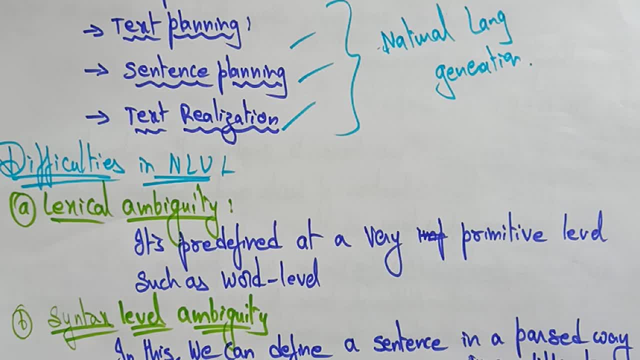 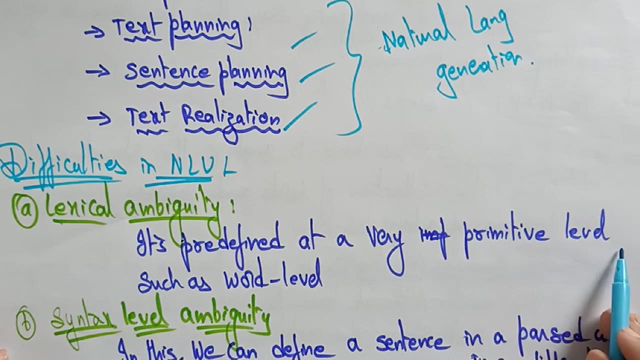 understanding and the generation. so to start the problem, first thing is you need to understand and then you need to generate. so some difficulties that are there in the starting step, that is, a natural language understanding. what are the difficulties? lexical ambiguity. it's a predefined it very primitive level, such 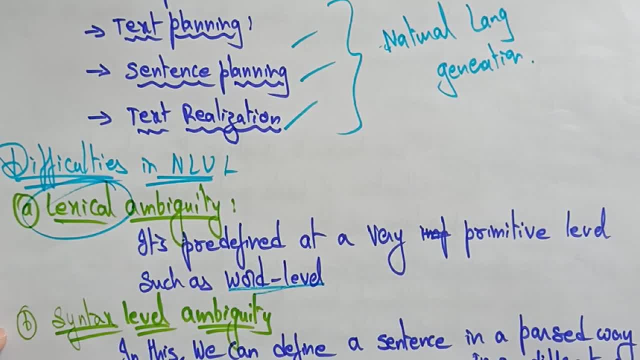 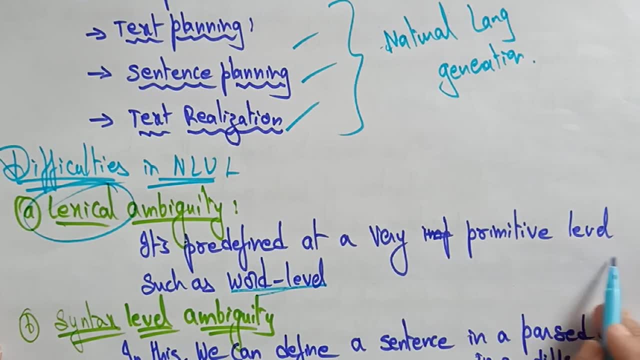 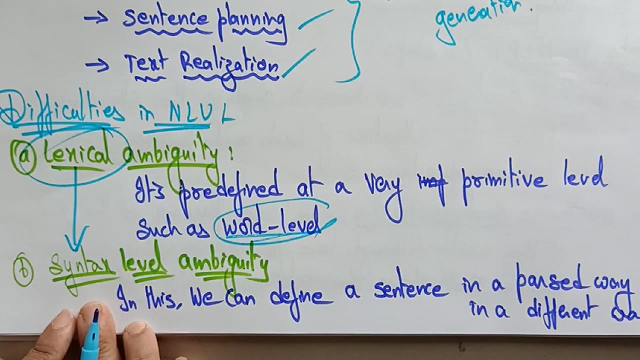 as word level. the lexical is a starting level of the conversion. okay, the system has, the compiler has a starting level. is a lexical level: okay, it's going to predefined it very primitive level, such as word level, and the next is the syntax level, after the lexical it has to convert it into. 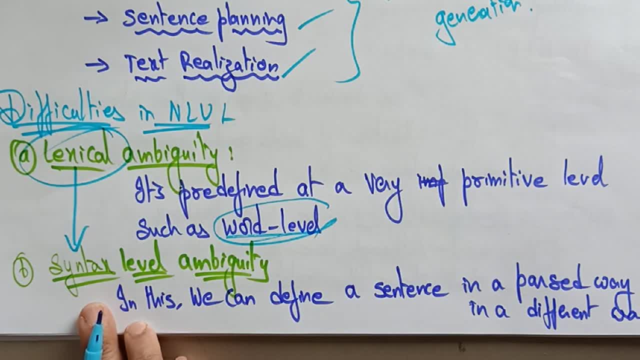 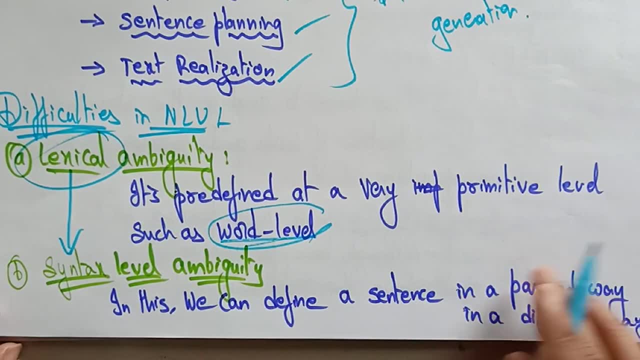 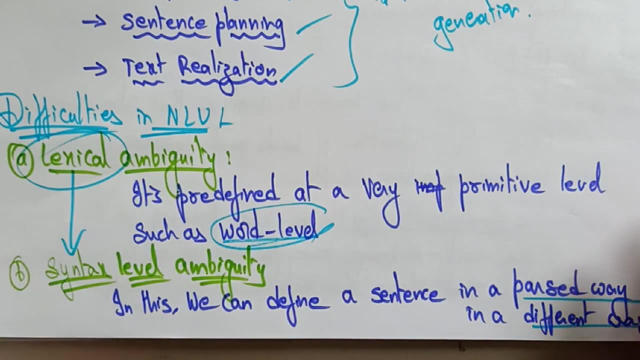 syntax level. so after every steps it follows, the final thing is a machine language it will become. then the system can understand the concept, the syntax level. ambiguity in this: we can define a sentence in a parsed way or different ways. so how you're going to represent the syntax level in just like 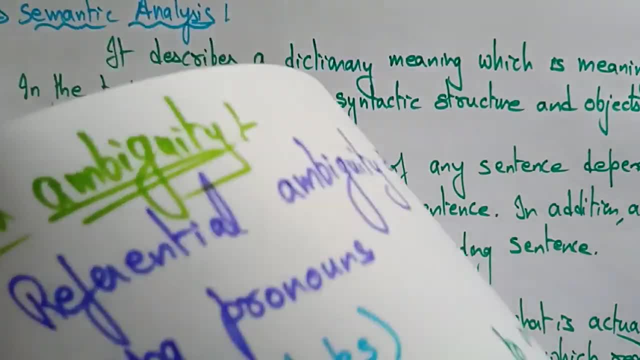 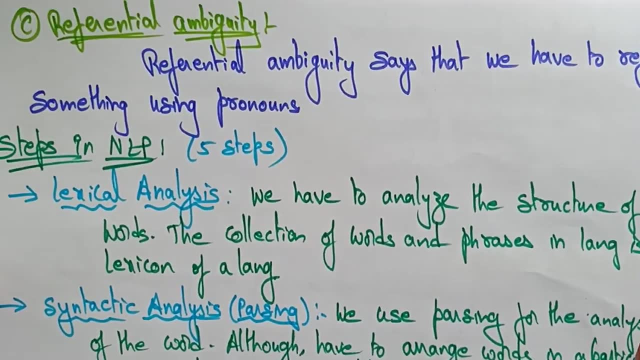 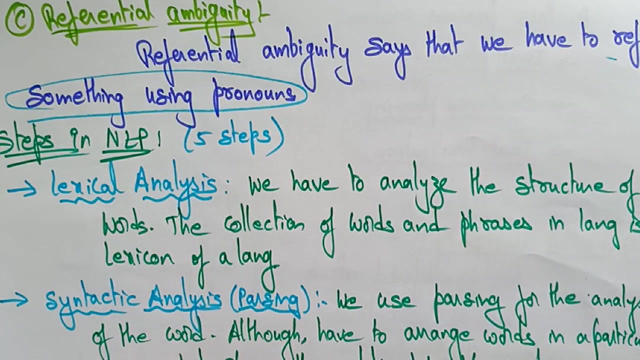 a parse tree, okay, or in a different ways we are representing. there should be an ambiguity in the parse tree also. Next is the referential ambiguity. Referential ambiguity means referential ambiguity says that we have to refer something using pronouns Okay. So these are all the difficulties of the natural language understanding. 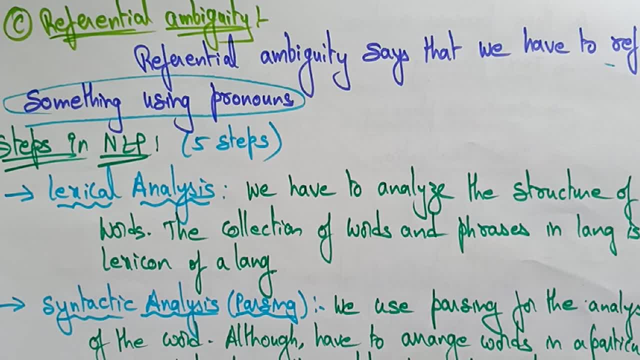 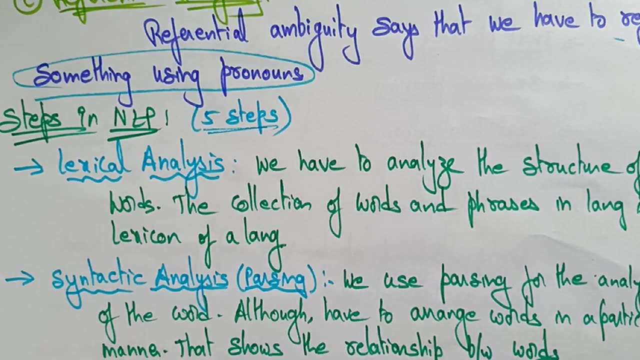 So first I want to tell you how you are going to implement this natural language process, step by step. So what is the step by step process to implement this natural language process? Let's see The there are total five steps are there to implement the natural language process. 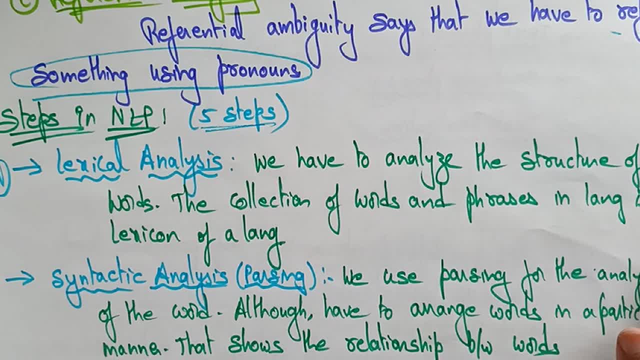 The first one is the lexical analysis. So, whatever I said, you have to take the input and you have to represent it. That is the first step of the compiler. We have to analyze the structure of the words. So the lexical analyzer is going to analyze the structure of words. 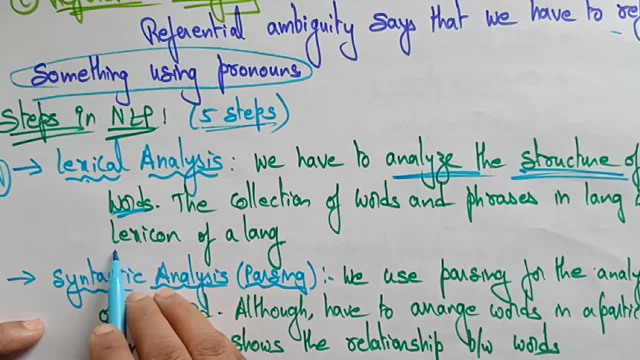 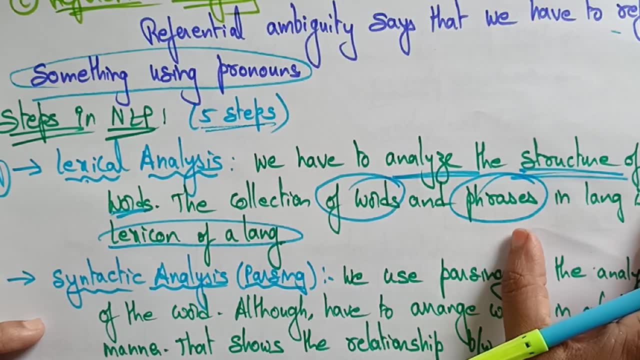 The collection of words and the phrases in a language is lexicon of language. The lexical analyzer is just taking the collection, The collection of words. what are the words are there and what are the phrases are there in a language that you call it as a lexicon of language? 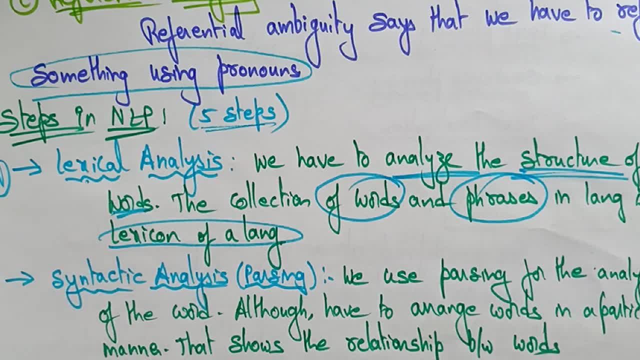 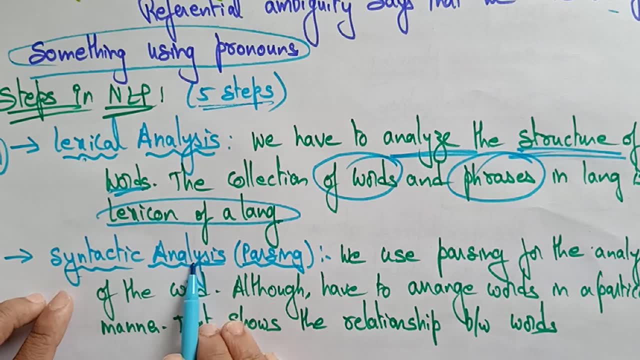 So first I analyze the structure of words and the phrases, what are present in my program. So the next step. So this is everything, the steps of natural language process. Next is syntactic analyzer. So in the syntactic analyzer I need to parse that. 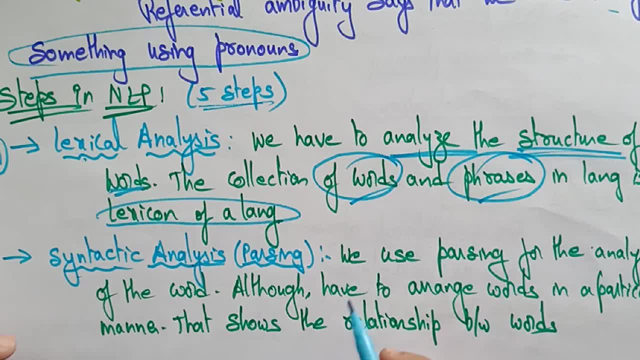 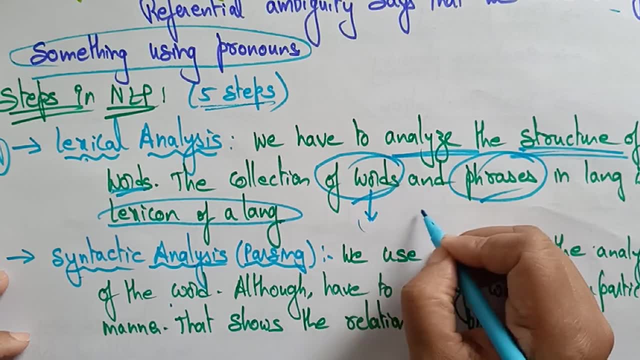 What are the words and the phrases that are present that I need to be parsed? Let's see. We use parsing for the analysis of the word, So whatever the word is there, Suppose some words are there- Hi hello, how are you? 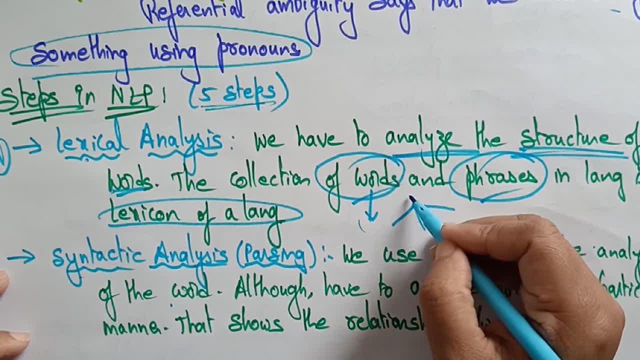 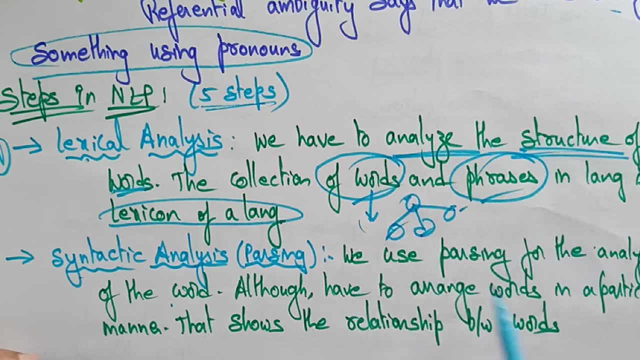 So that I need to be represent in the parse. I need to parse that, I need to parse that words. That is, we are analyzing the each and every word in the phrases. We use parsing for the analysis of the word, Although how to arrange words in a particular manner that shows the relationship between the words. 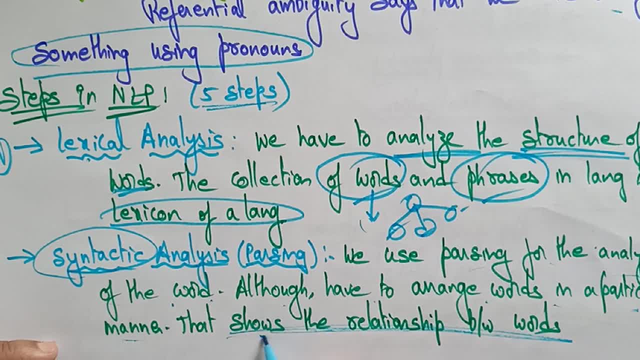 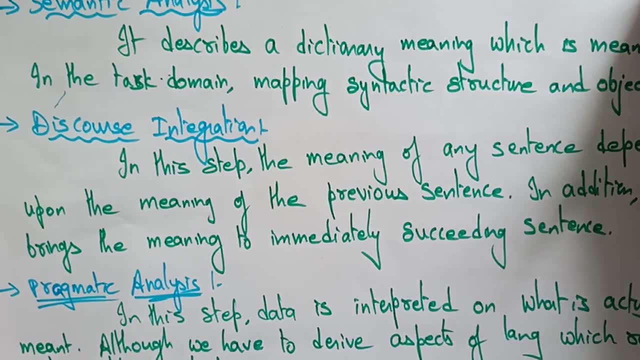 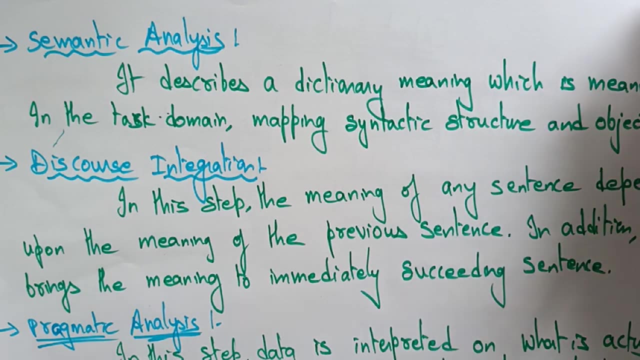 So this syntactic analyzer, what it is doing? So it is just showing the relationship between the words by parsing, Parsing to each and every word in the phrase. So the next step here is the semantic analysis, analysis, So lexical analysis. over that is the analysis analyzing the structure of words. 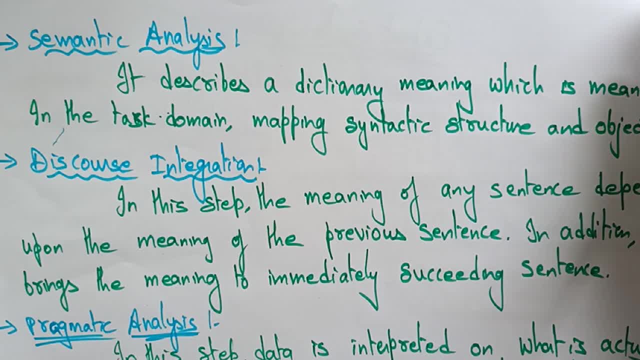 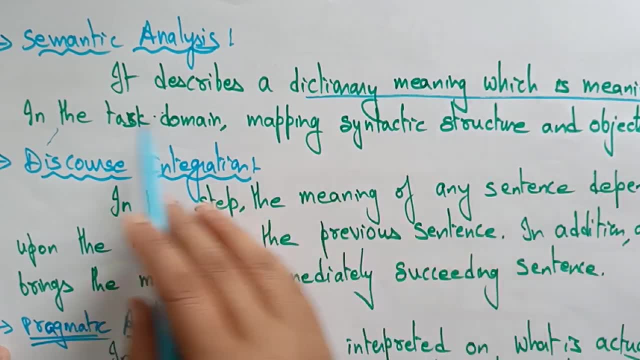 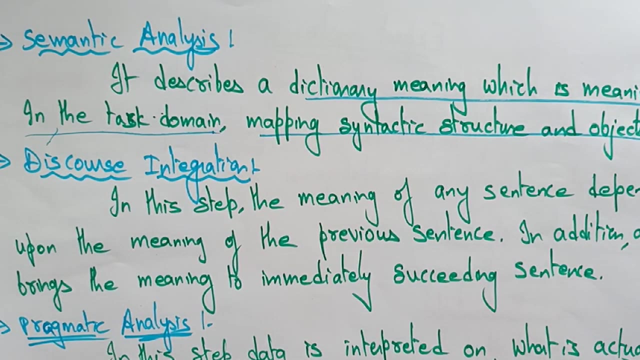 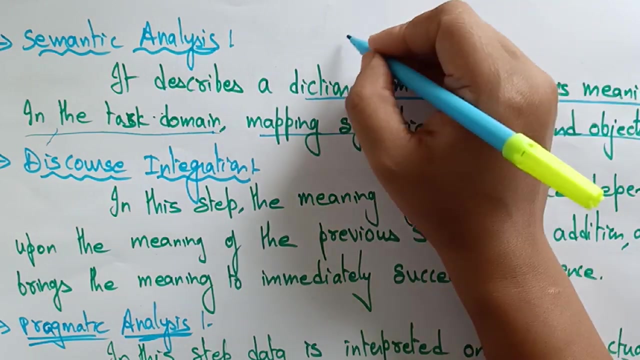 Next, syntactic analysis is over, That is, we are showing the relationship between the words. Next is a semantic. Semantic: it describes the dictionary meaning which is meaningful in the task domain mapping syntactic, structure and object. So, after showing the relationship, I need to know the word of meaning of each and every word so that the so in the Google suppose you are giving something like a document, you are giving just like a doc. 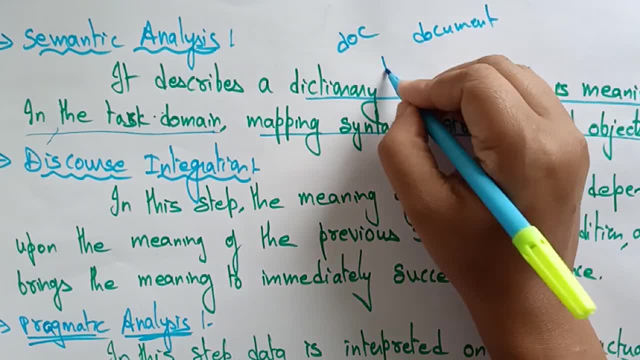 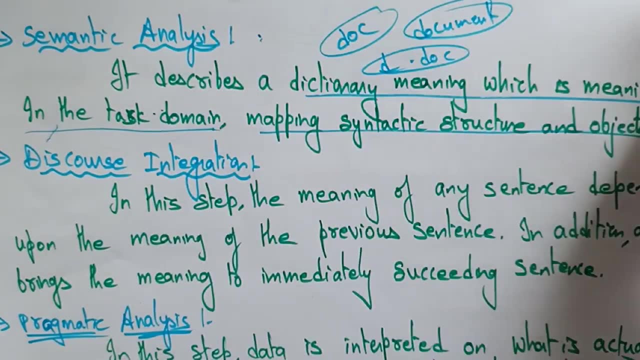 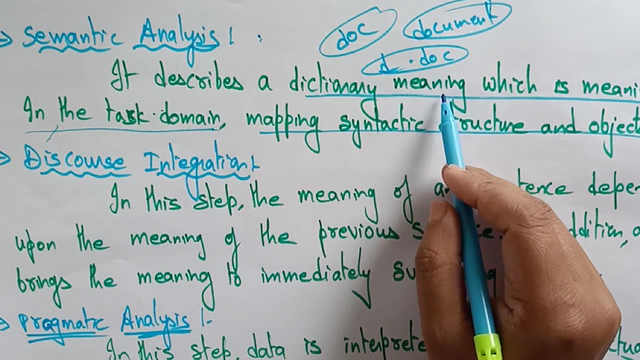 Some people will give the full name as a document. Some people will use a dot- divorcee. like. the different formats will be there. The same name is having different meanings will be there so that everything should be maintained by. in the semantic analysis, It describes the dictionary meaning.